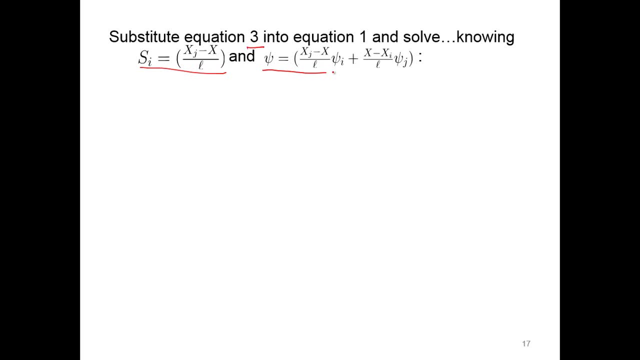 and the length and we have our psi is the shape function of node i plus the psi of node i plus the shape function of node j times the psi of node j and we can substitute those in and what happens is right. here is the expansion of that first second order term. so we have this term and this term of the second order derivative, and then we have the other. here's the first order. 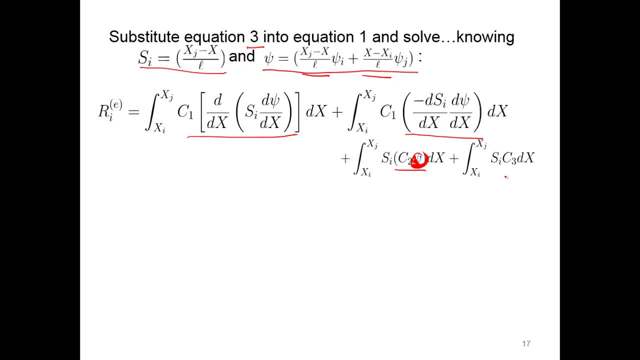 oops, first order of psi there and then the third coefficient: alright. so if we integrate these guys out, we come up with this term alright, and ooh, look at that, like those two guys are going to cancel themselves out, alright. and then we have term down here: c1, alright, actually we got x1, xj. 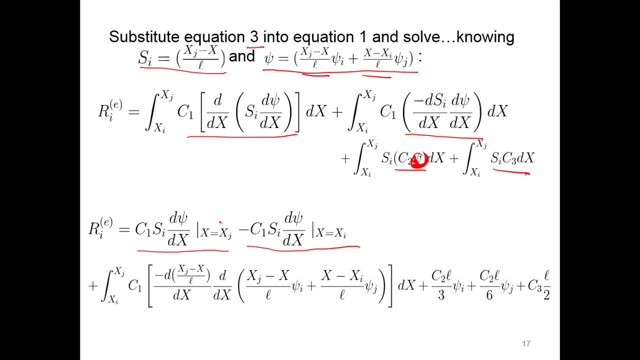 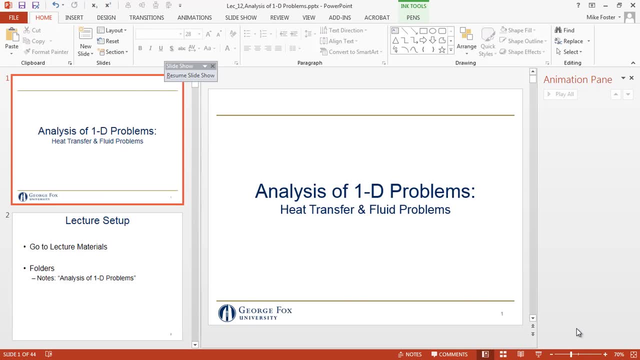 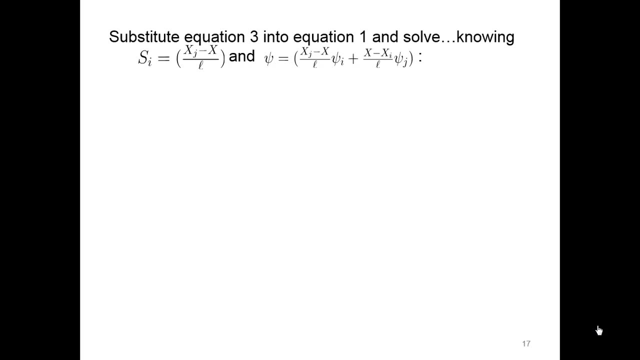 alright, I want to write up some equationache here. ok, so we're going to substitute equation three- that was the one at the bottom of the previous slide- into equation one. so equation one was the one, for equation four was: equation three was the one for equation one, and then equation- why is? and then wait for equationhe has to be really powerful, So we can substitute equation two and equation three is the first advantages of taking vale two, because it saves us somewhere, right? 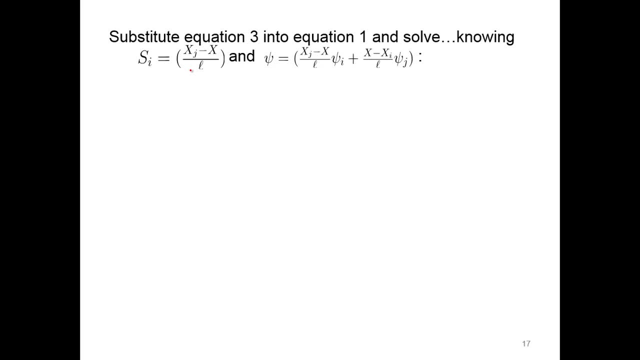 the residual at node i In Solve, knowing that we got the shape function at node i and we have this expanded here- form for finding psi at any location in our element. So the residual at node i becomes: here's our first term. So we've expanded our second-order derivative. 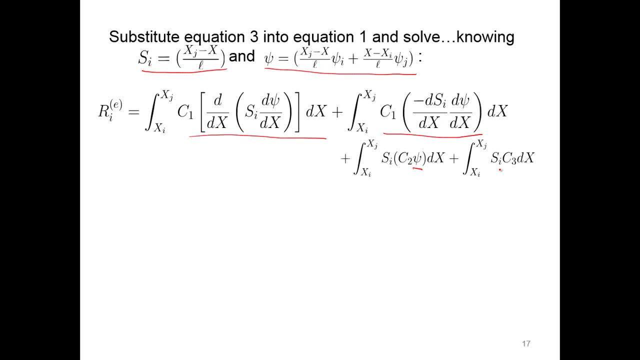 into these two terms. Here's our first-order term for psi and then here's the coefficient of three. So here what we've done is we've gone through with the integration of this first term. So going through that integration of the first term. 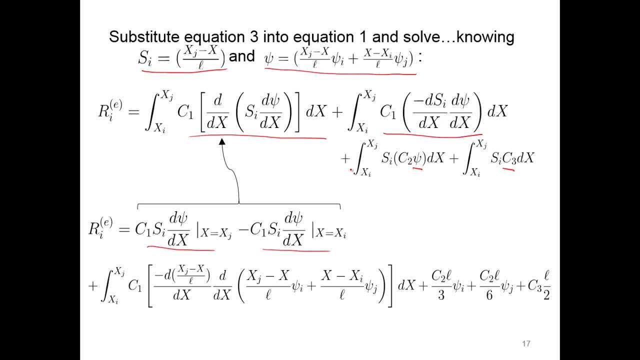 creates these two terms. The second term's been expanded. so what? we've substituted for psi right here, and that's where we get everything here. that's in parentheses. So we did the substitution of psi which is up here at the top, And then for the shape function at node i. 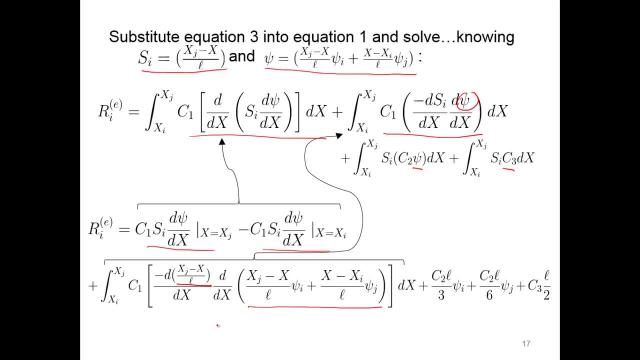 that's what's right here. So that's the shape function at node i. we've substituted here, We'll put it in there. And then the last two terms here, or three terms. the first two are from the integration of the first-order psi term. 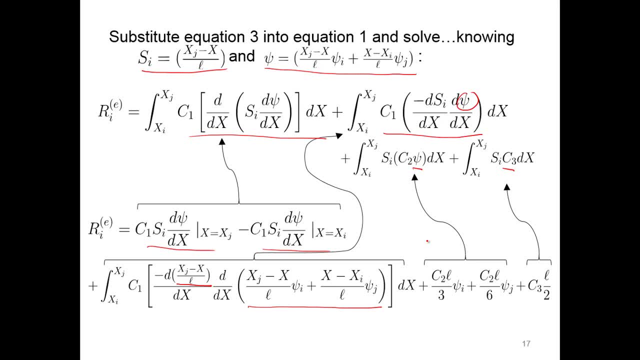 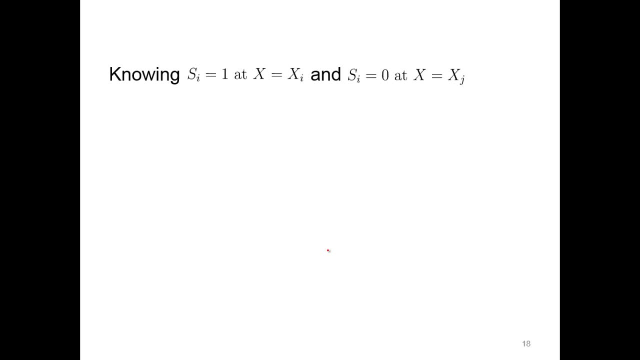 and then the last term, there is the integration of our coefficient of three. So we're gonna make a substitution here, And so we go back and forth if we need to. So we know the shape function at node i is one at node i. 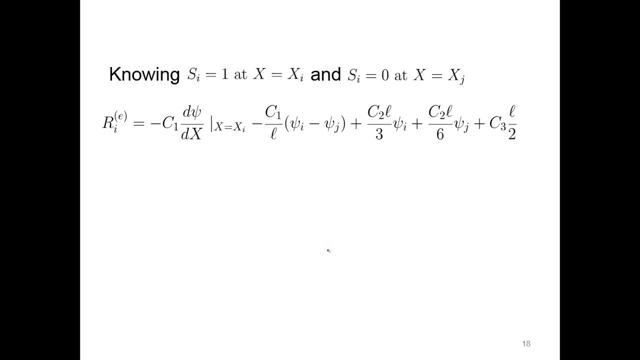 And shape function for node i is zero at node j. So knowing those two we can plug in and we can solve this one further. So we get the psi of node i minus psi of node j for that function there, And then these guys are pretty much. 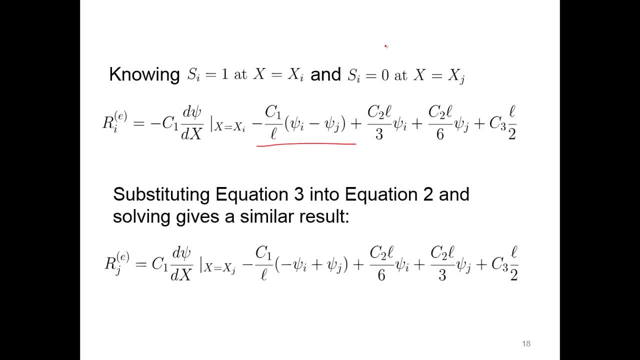 what they were on the previous slide. We can do the same thing. So equation three was the second-order expand second-order into first-order derivatives And equation two was the one for the residual at node j And equation three was the one for the residual at node j. 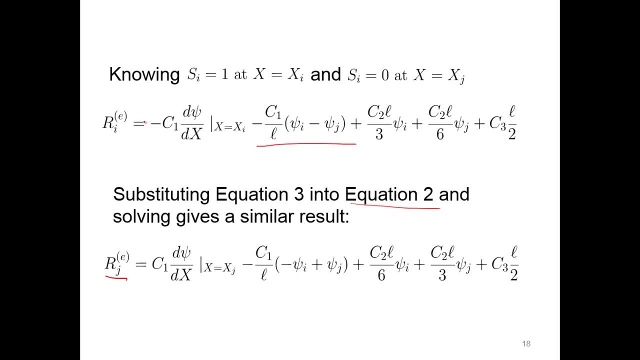 And equation two was the one for the residual at node j, And equation three was the one for the residual at node j, So we get basically a very, very similar form. So here's residual node I up here and a residual node J down here. 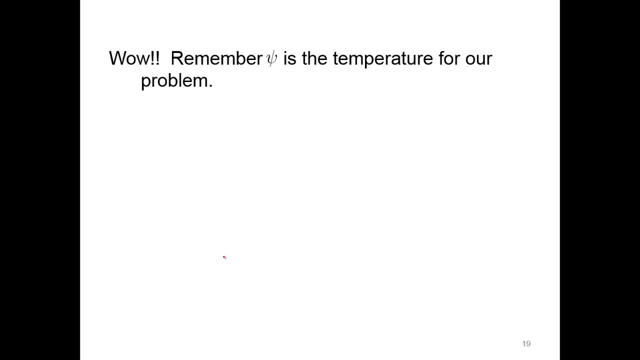 We're gonna take those and we're gonna put those in a matrix form. So, remember, psi is the temperature or can be the temperature for our problem. So we're gonna assemble this in a matrix form. So here are the two residuals here. 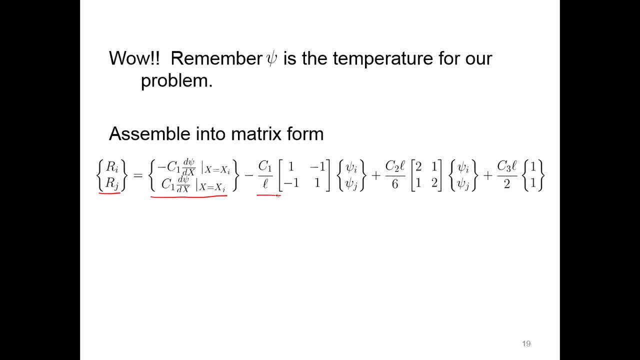 Here's the first part of that second-order derivative. Here's the second part of that second-order derivative. This is that first-order term. and then here's that, the last term there, the third coefficient. All right, so setting the residual equations to zero. 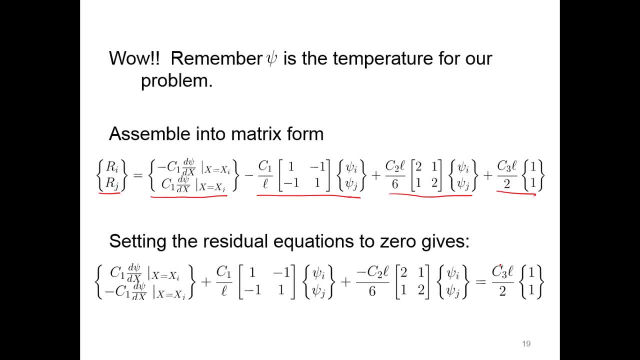 so if we set these two guys equal to zero, we can isolate this guy- this last term by itself equal to all the rest of the terms. So again, that's a lot, but again we're gonna go back and get more sense of what's happening. 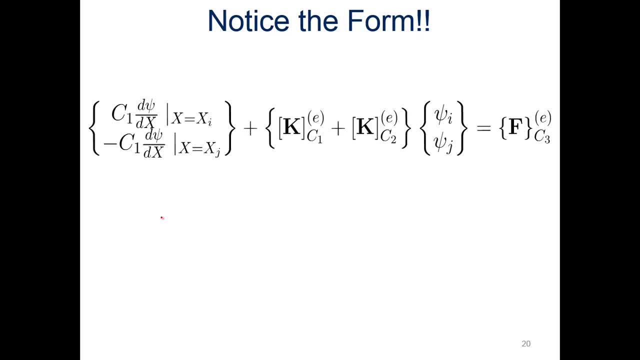 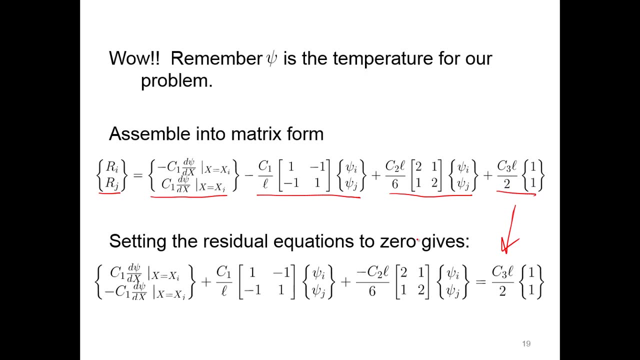 but I wanted to see it from a general term, and then we'll go back to that. So notice the overall form here, though. So I'll go back real quick one slide. So notice what we got here. This looks kind of familiar, right. 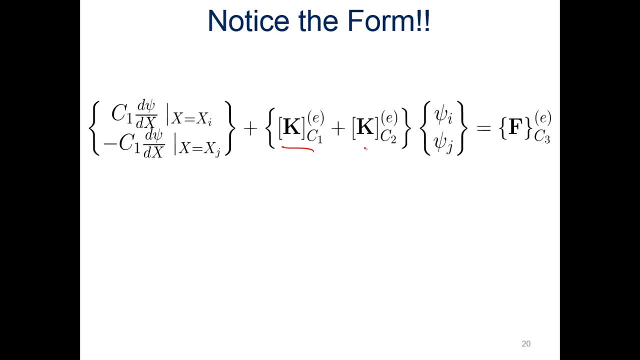 This equation? All right. so we have these two. what looks like stiffness matrices? All right. what do we got over here? Contributes to the element conductance and load based on the boundary conditions. All right, so that's the second-order term. 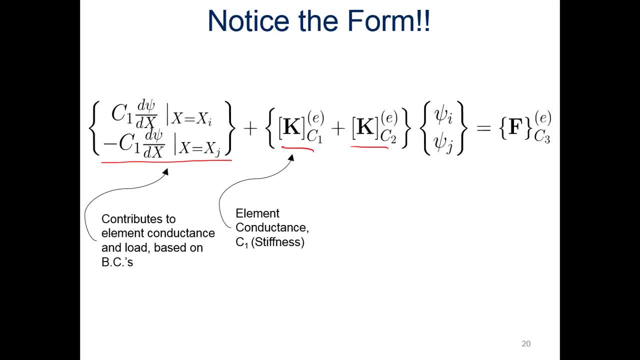 so that makes sense, contributes to the conductance. All right, this is the element conductance. or you can think of it as a stiffness right, The stiffness matrix. This is also the element conductance, but in this particular problem. 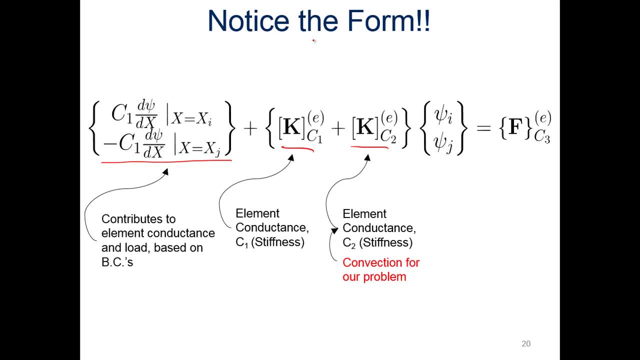 it's convection. for our problem it's a convection term. And finally, we have a thermal loading. So for a while we had a load matrix due to force in our structural analysis, In our thermal analysis, it's a thermal load. 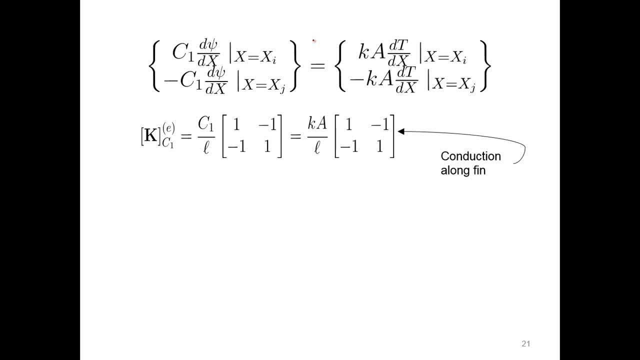 All right. so looking at that first term, all right, what we've done here is we've substituted in. let me go back here. we've substituted back in for C1, substituted in our KA. so for our first term there. 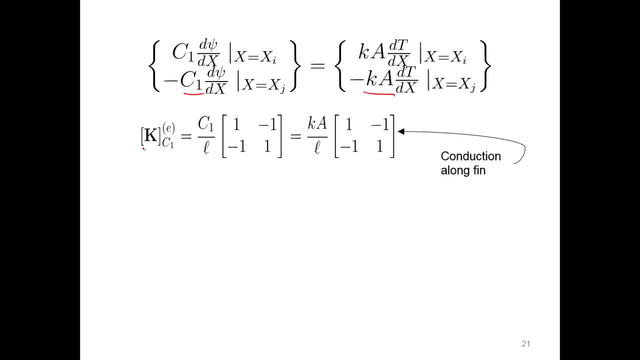 All right, so for our stiffness term. all right, so our first stiffness term for C1, we're substituting back in KA, just as we did up here, And this is the conduction along the fin. All right, so. conduction coefficient times area. 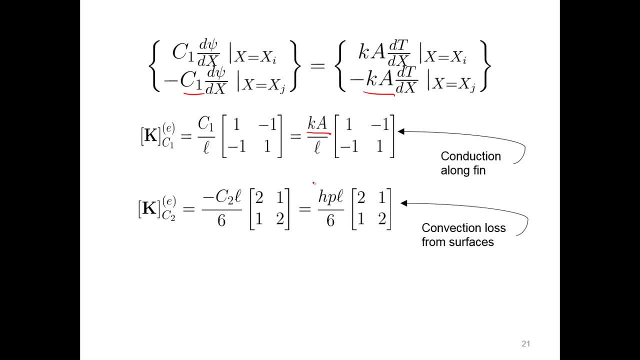 over length. And then we have these stiffness values in here. So the concerns of conduction along the fin, right conduction along the fin This next term, we're still standing back in for C2, or H times the perimeter. 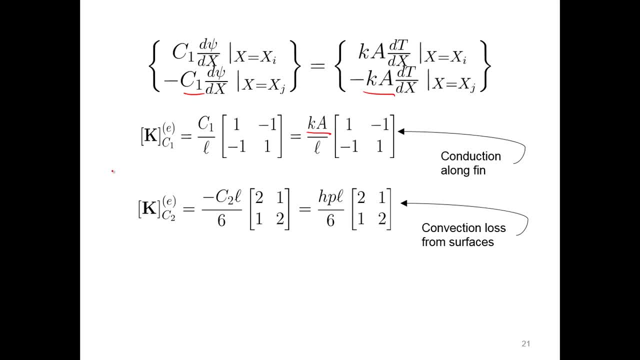 This is the convection loss from the surfaces of the fin. So if we're going down the fin and the fin's like this, we're going this way right. This second matrix up here refers to the convection loss along the surface as we move along it. 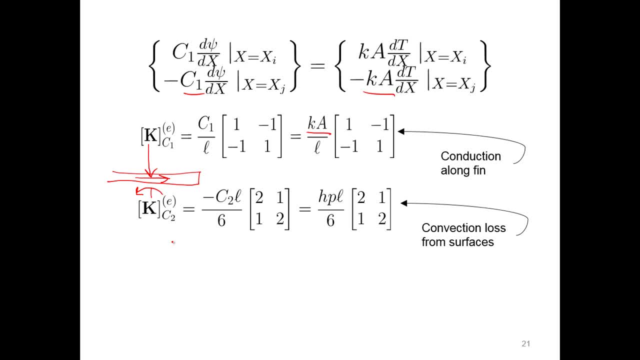 Whereas this one refers to this conduction along the fin And this last one is the convection load from the fluid. all right, So it's a load from the tip, so it could be a tip condition. All right, So assuming a third boundary condition, 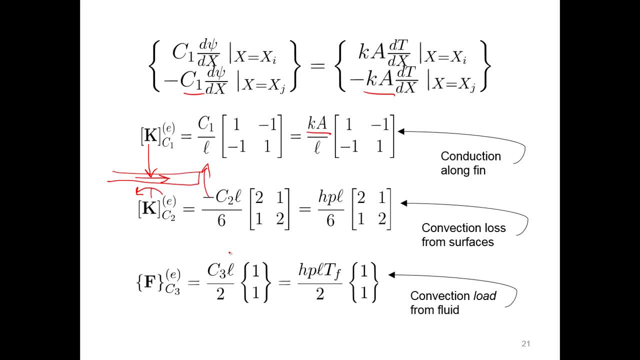 Oops, All right. so it's a load force against the body hours where you have sideburns, and this is a load. And the third boundary condition we're gonna have to be people from the left side, which is 말�is. 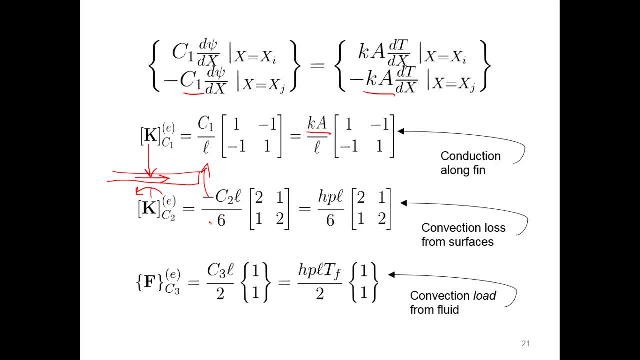 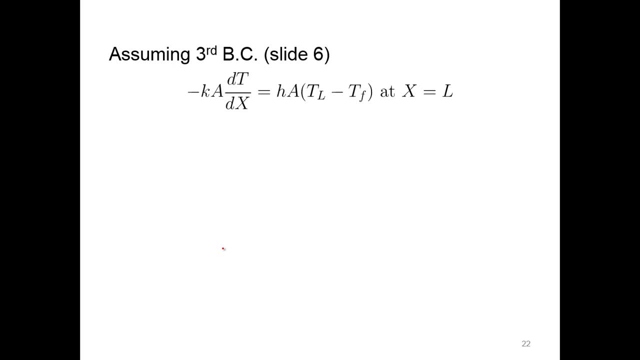 in the third boundary condition. So basically, we're out of the difference between two orders. now we're in a verticalे search老 and br- and it helps to see how the spread. okay, Let's look at the share and share- same table. 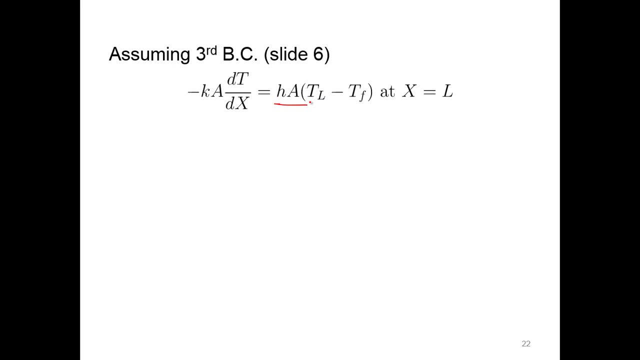 So we had two positions, so basically ran through the door And then characteristics of theанич part of the system is that it takes the flow against the temperature. We let our sp stiff. we created our障, which makes sense at the end of our fin. 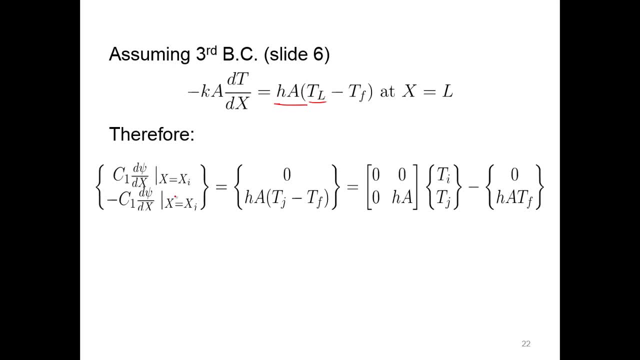 So therefore, if we put the equation together here, we have a conduction that would happen into the tip, we would have convection from the tip and we'd have these other terms, all right. So basically, what we're doing here is we're looking at. 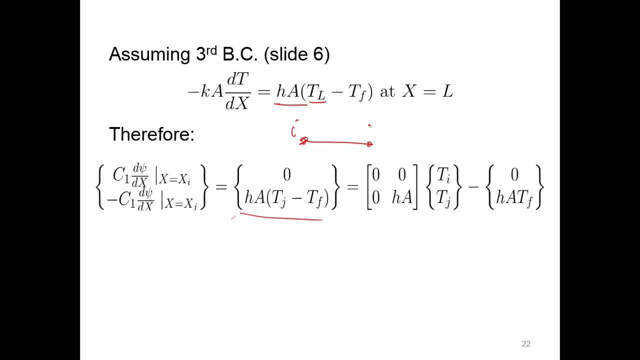 if we had an element here. we have node i and node j and if j was at the tip, it would be the one that's interfacing, having the convection at the tip. So that's why there's no terms here, just equals zero at node i. 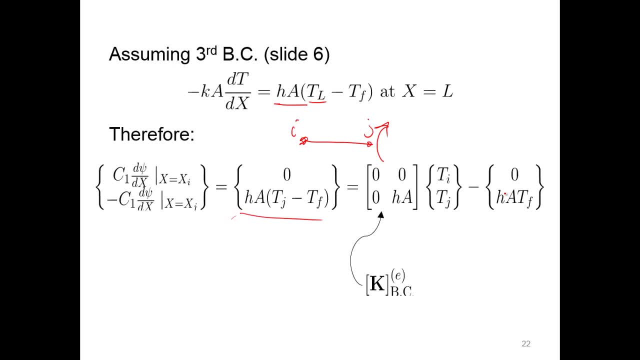 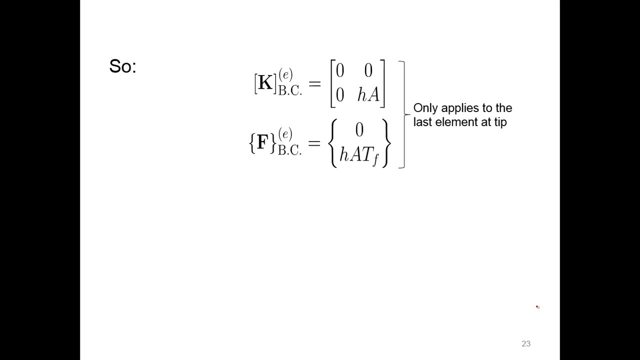 and then we have convection here for all the j terms. So there's the boundary condition, all right, Boundary condition for the convection matrix, and then a force function because of the temperature in the fluid. So both those only apply to the last element at the tip. 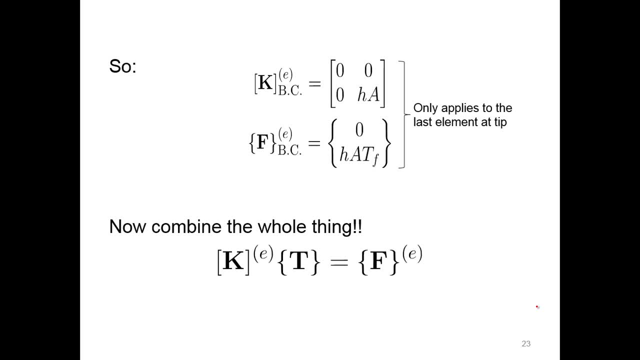 because that's where that shows up. we have the convection from the tip, All right. so let's combine the whole thing together. We got our stiffness, we got our temperatures and we got our forcing functions, All right. so only for the tip element. 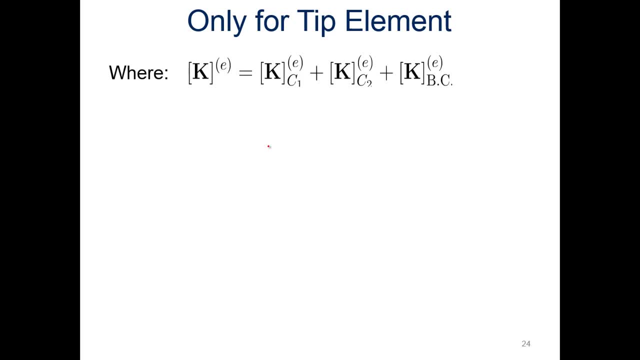 we combine all three of these things, where we have our first stiffness matrix and our second and our third boundary condition matrix, All right, so in that case our total element stiffness contribution is one from conductance, one from convection to the side. 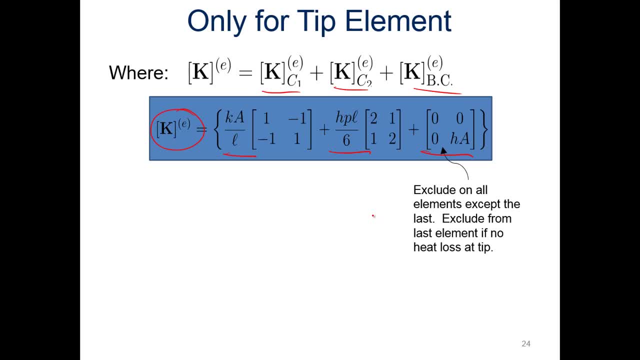 and one from convection from the tip. So on all the other elements we exclude this one, except for the tip. all right, So exclude from all the last element if no heat loss from the tip. So if we don't assume convection to the tip. 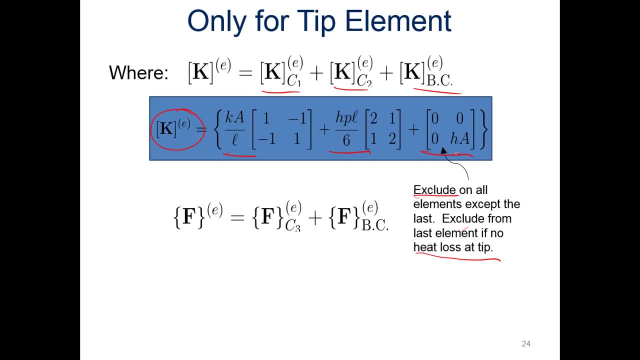 then we exclude this. So again, we'll get practice with this. I'll show you how this works. All right for the forcing function. again, you wanna include the C three term that we already had, and then we also have boundary condition. all right. 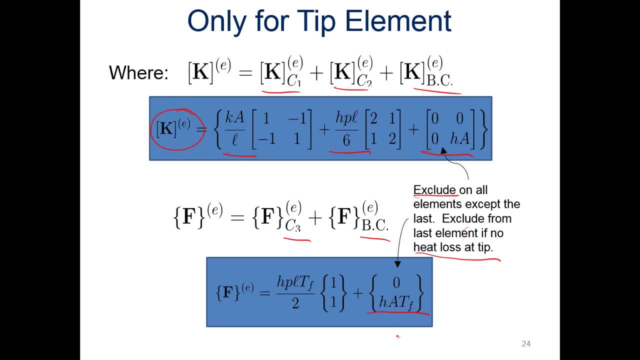 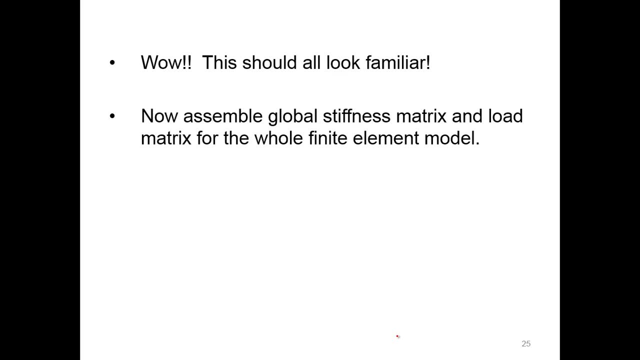 So we're gonna exclude this one as well if we don't have convection from the tip. All right, so okay, hopefully this all looks familiar, All right. so we're gonna again from kind of the stiffness perspective. now we're gonna assemble a global stiffness matrix. 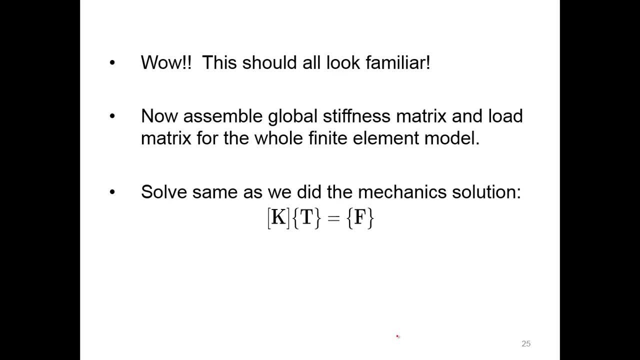 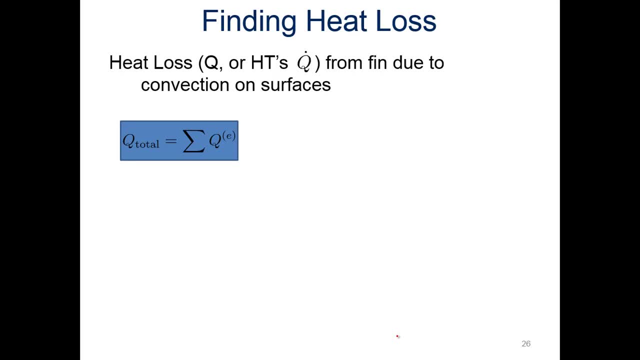 All right, so you can find more examples in textbooks and online to give you other examples. All right, so you can find more examples in textbooks and online to give you other examples. I also see cheese transfer and for heat transfer I use Q dot, so rate heat transfer rate. 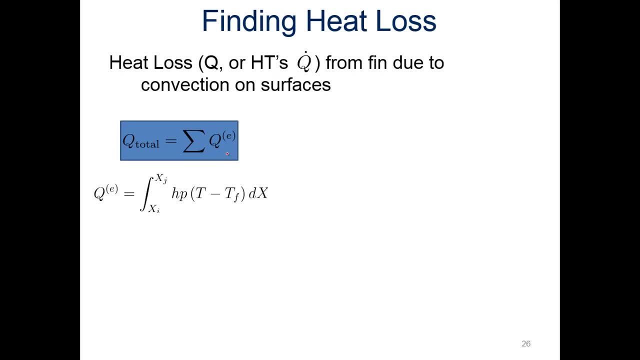 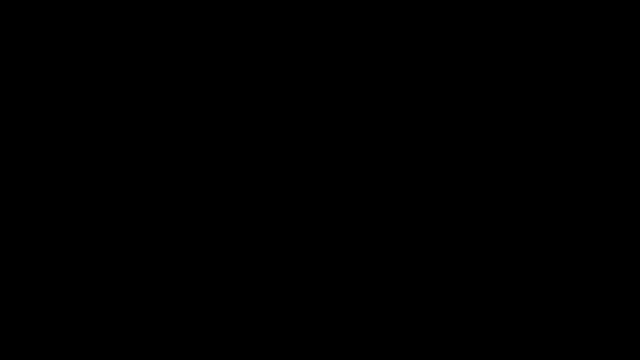 So, due to convection on the surfaces, basically we need to sum the Q dot that happens through all the surfaces. So here's our convection Q dot equation. so HP, we don't have area here because we're gonna integrate along the X direction. 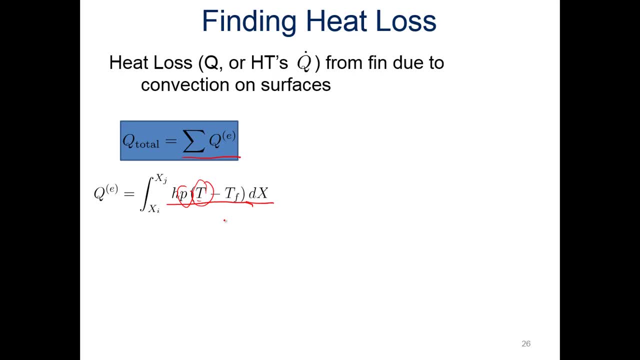 so it's just the perimeter, And then we have the temperature of our surface minus the temperature of the fluid. So, substituting in for the temperature equation, that's what's coming in here. So substituting in here the shape, function, form of our temperature, that's substituted in there.